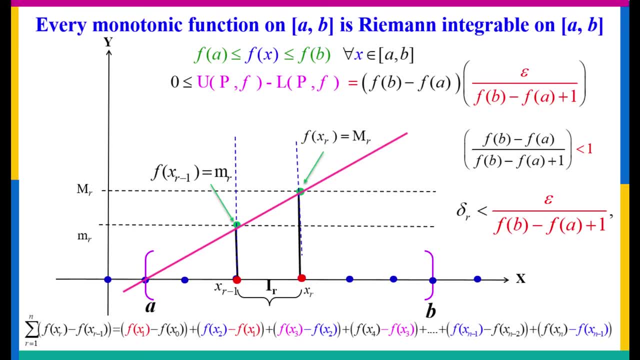 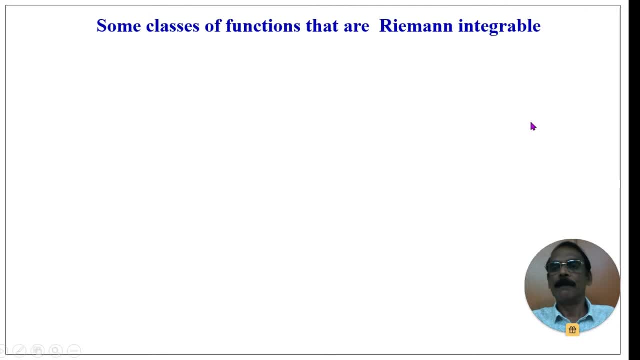 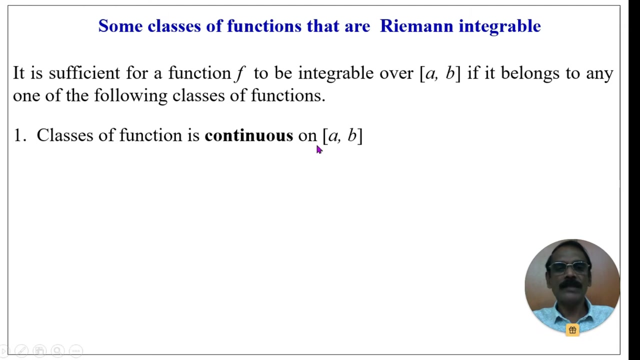 Some classes of functions that are Riemann integrable. It is sufficient for a function f to be integrable over the closed interval a- b if it belongs to any one of the following classes of functions: Classes of function is continuous on the closed interval a- b. Classes of functions: monotonic on the closed interval a- b. 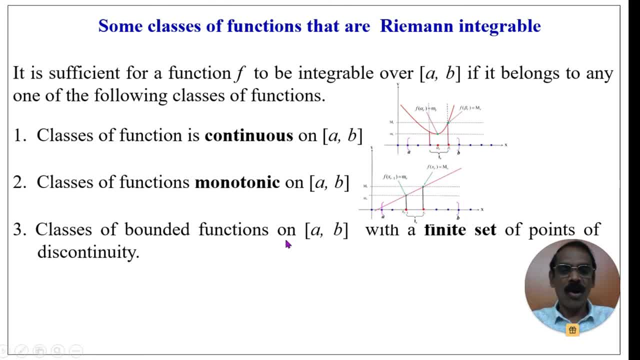 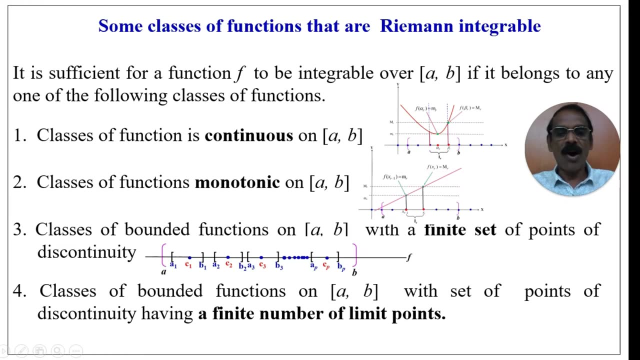 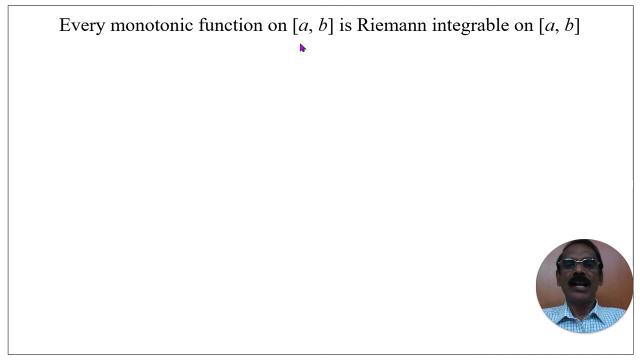 Classes of bounded functions on the closed interval a- b With a finite set of points of discontinuity. Classes of bounded functions on closed interval a- b with set of points of discontinuity having a finite number of limit points. Every monotonic function on the closed interval a- b is Riemann. 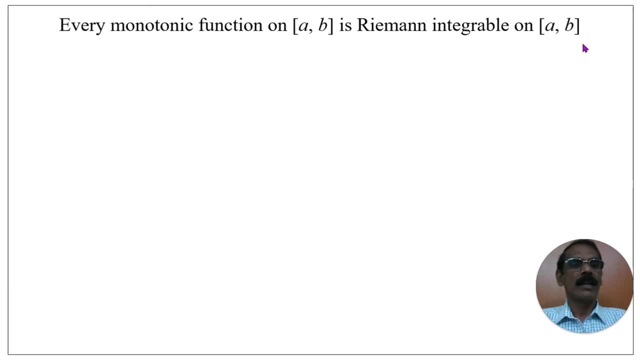 Riemann, integrable on the closed interval: a: b. Proof. We know that a function is said to be a monotonic function if it is either increasing function or decreasing function. Therefore, we will be having two cases here. One is for increasing function. The case number two will be for decreasing function. 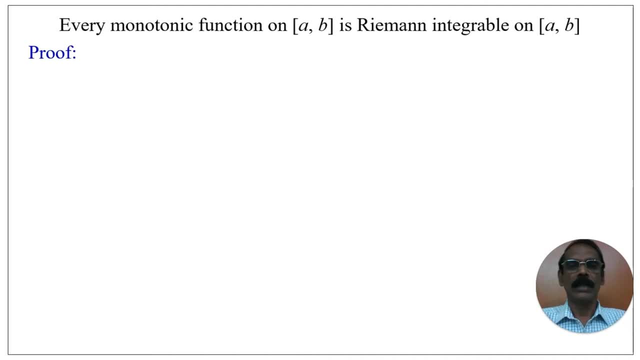 Therefore, to show That every monotonic function is Riemann integrable, We have to show that increasing function is Riemann integrable and the decreasing function is also Riemann integrable, And hence we can conclude that every monotonic function is Riemann integrable. on the closed interval a- b. 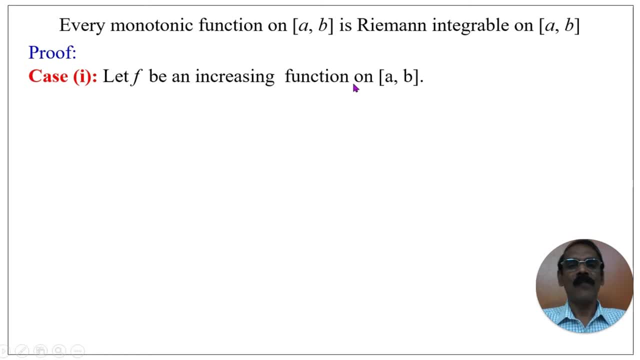 Case one: Let f be an increasing function on the closed interval a- b. Therefore, a is less than or equal to b implies f of a is less than or equal to f of b. This is the definition of increasing function. As the values increases, its functional value also increases. 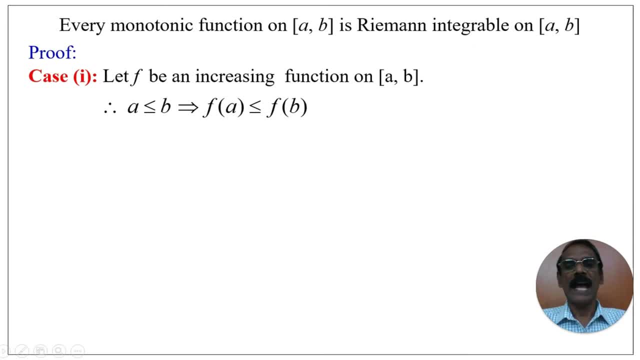 Therefore, the function is an increasing function and this is the condition for increasing function, That is, f of a lesser equal to f of x, lesser equal to f of b, for all x belong to the closed interval, a comma b, That is, f is bounded on the closed interval, a comma b. That is the value of f of x. 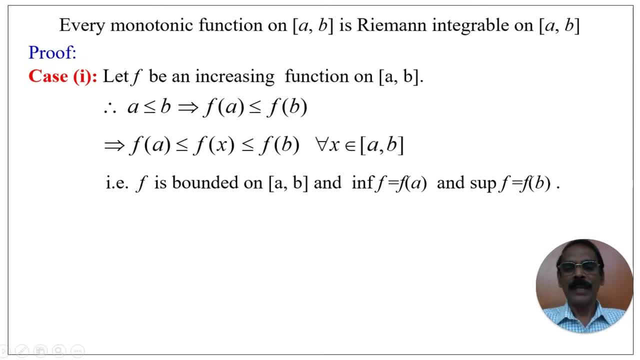 is from f of a to f of b. Therefore it is bounded, and infimum of the function f is f of a and the supremum of the function f is f of b. Let epsilon be greater than 0 and p equals to the set consisting of the points x not equal to a comma, x1, comma x2, so on xr minus 1 comma xr. so 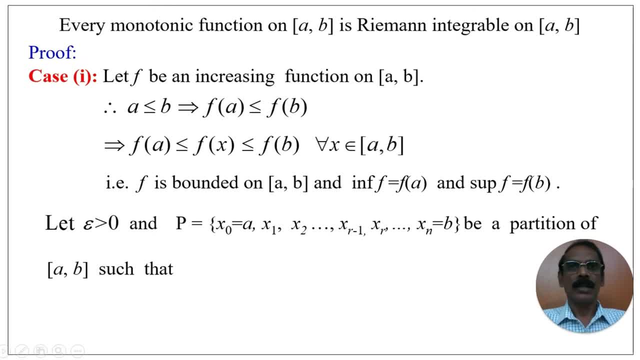 on xn equal to b, be a partition of the closed interval a comma b, such that delta r is less than epsilon by f of b minus f of a plus 1, where r is equals to 1, 2, 3, so on n, let us call it as 1.. Let small mr and capital mr be the infimum and supremum of f in ir. then 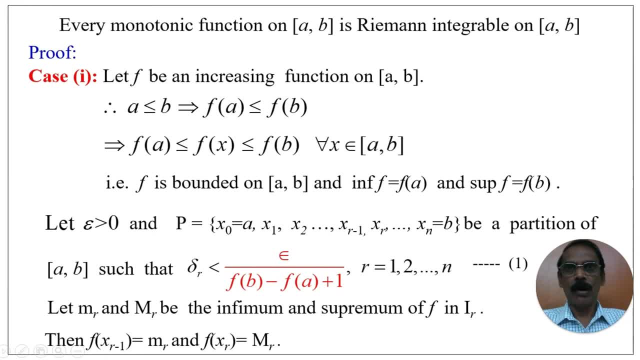 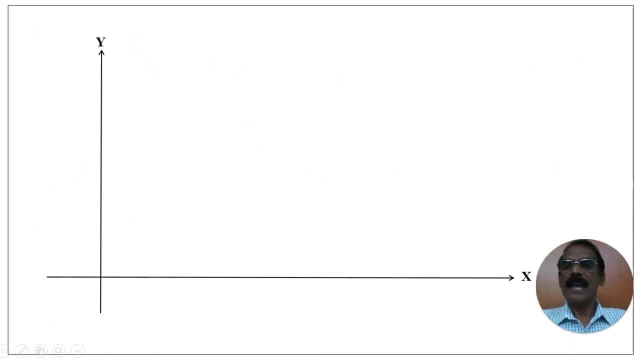 f of xr minus 1 is equals to small mr and f of xr is equal to capital mr. This is x axis, y axis. consider: this is a function which is an increasing function. this is a closed interval, a, comma b, and these are the points. let us consider the rth subinterval ir. this is xr. 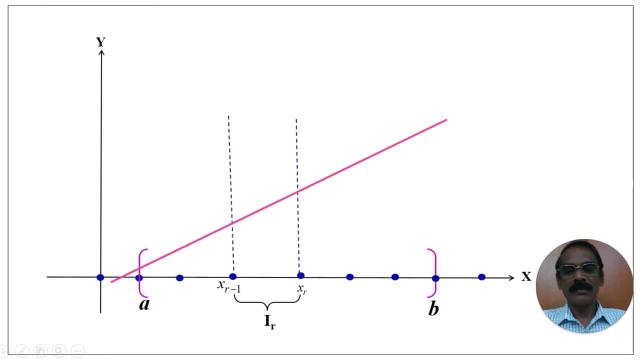 minus 1, this is xr. so this is the interval ir. if you consider the part of the curve in this closed interval ir, The minimum value is here. the maximum value is here. the minimum value is the value of the function at xr minus 1, so this is the minimum value, mr, in the part of this function, in this. 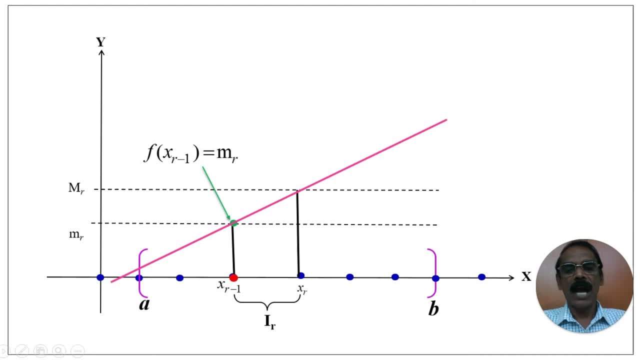 interval ir. the greatest value, the highest value, are the supremum of the function f in the interval ir is this point, that is, nothing but the value of the function f at xr, which is equal to capital, mr. now look at the comparison. this graph represents a continuous function. 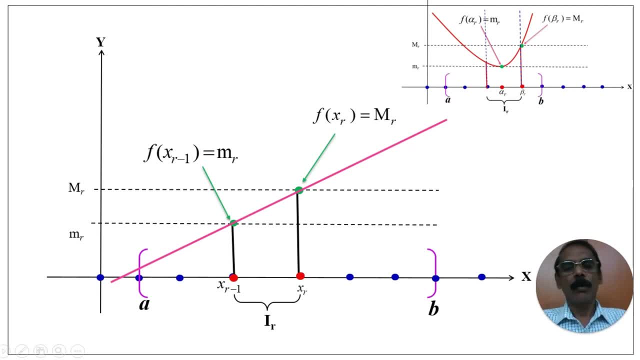 this function represents monotonic function. the difference is the infimum and supremum in the rth subinterval of the function. f may be anyway. in this continuous function, Infimum small mr is equal to f of alpha r capital mr is the supremum of the function f in the 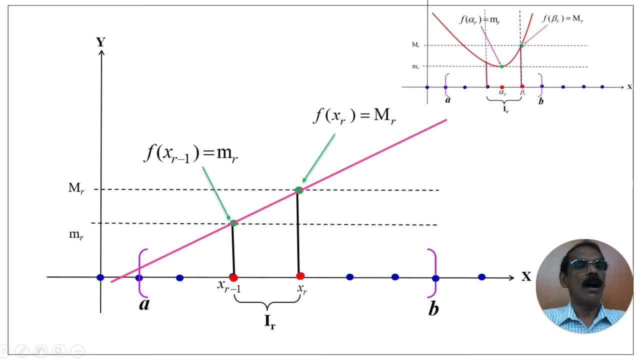 interval ir that is equal to f of beta r. and remember that alpha r and beta r need not be the n points of the interval ir, whereas in the case of increasing function, those points, namely here alpha r stands for xr minus 1, beta r stands for xr, and these two points, xr minus 1, xr, must be the 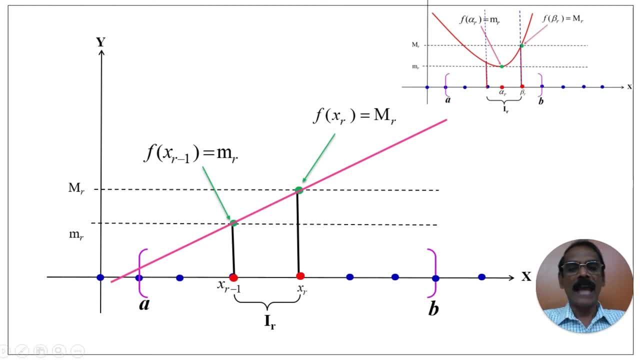 n points of the subinterval ir. here alpha r and beta r need not be the n points of the interval ir, Whereas, except alpha, xr is equal to f and xr. for the interval ir anyways, we cannot as n points of ir, whereas xr and xr minus 1 must be the n points because it is a increasing function. 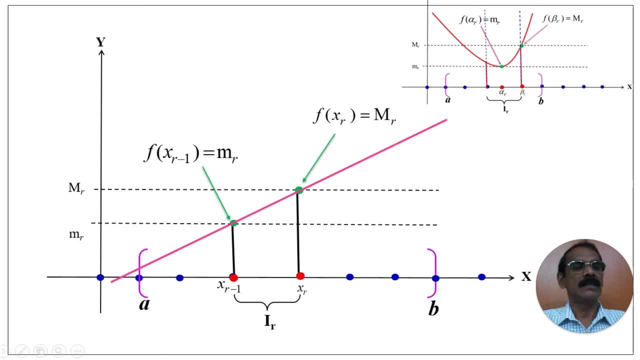 whereas if we see the continuous curve, it is neither increasing nor decreasing, because here it is decreasing, then it is increasing. therefore, the two points, alpha r and beta r, may be from? hmm, definitely xr minus 1 to xr. 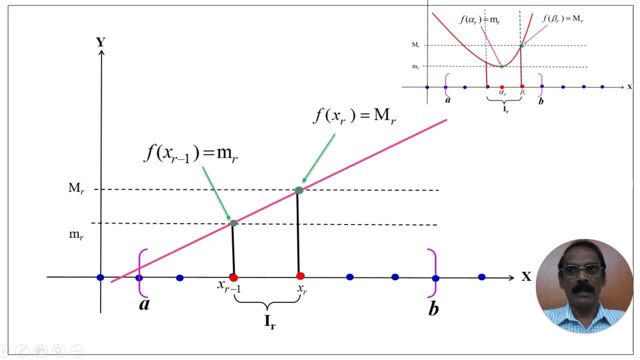 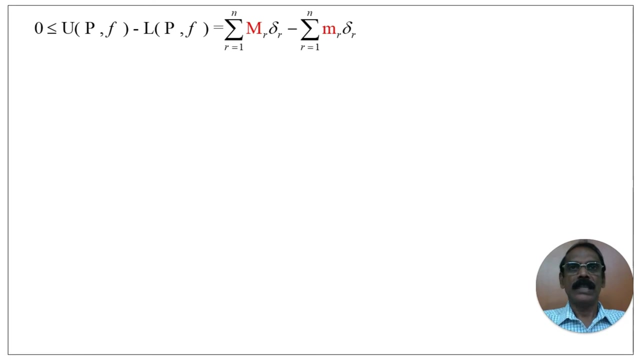 The infimum must be the value of the function at xr minus 1.. Here the supremum is the value of the function at xr, where xr minus 1 and xr are the end points of the interval ir. Now our aim is to show that the given function f, which is an increasing function, is Riemann integrable. 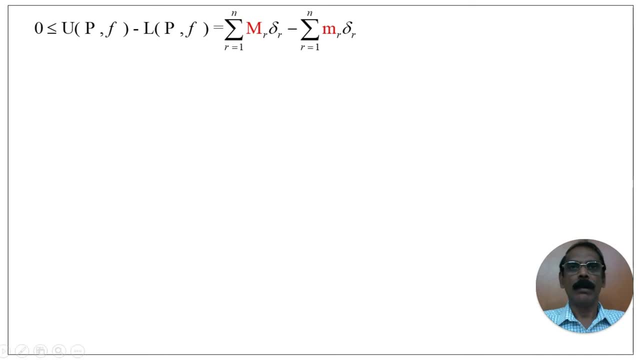 To show that the function f is Riemann integrable, we have to show that the difference of upf and lpf is less than epsilon. Therefore, consider u of p comma f. The value of u of p comma f is sigma R equal to 1 to n capital M R into delta R. minus l of p comma f is sigma R equal to 1 to n small m R into delta R. 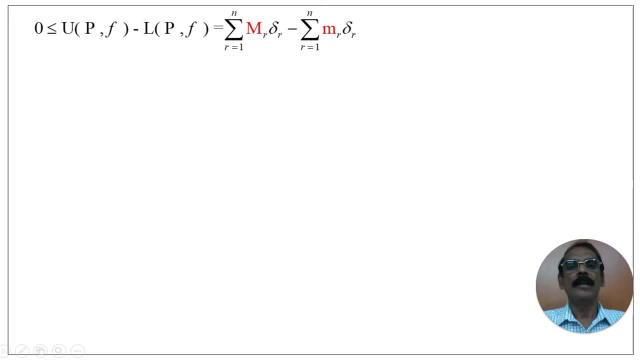 Where small m R and capital M R are the infimum and supremum of the function f in the rth subinterval And delta R is the length of the rth subinterval That is, equals to sigma R, equal to 1 to n capital M R minus small m R into delta R. 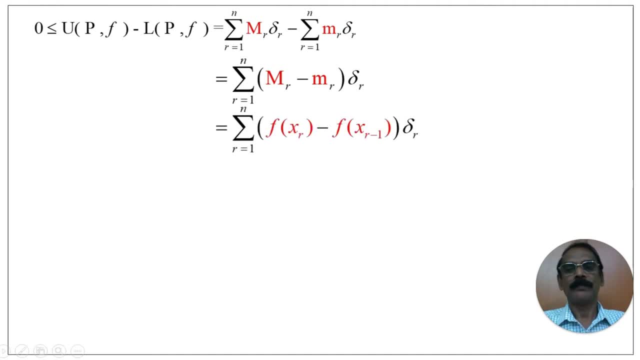 That is, we have taken delta R out, That is, equals to sigma R, equal to 1 to n f of xr minus f of xr minus 1, into delta R, Because the value of capital M R is f of xr. The value of small m R is f of xr minus 1.. 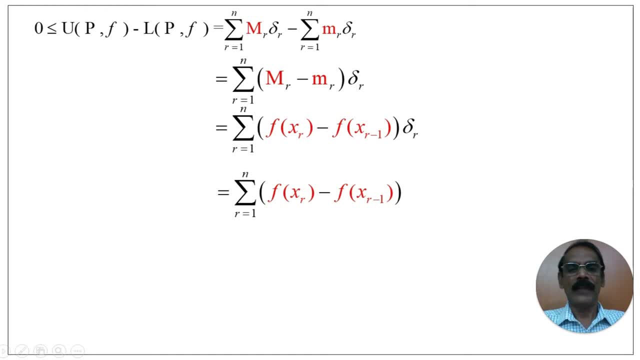 That is equals to, That is equals to sigma R, equal to 1 to n f of xr minus f of xr minus 1 into delta R. What is the value of delta R? Delta R value is less than epsilon by f of b minus f of a plus 1.. 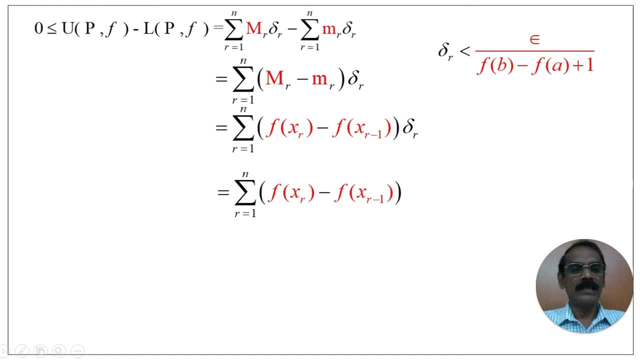 Therefore, now we are going to replace the value of delta R, which is less than epsilon, by f of b minus f of a plus 1.. Therefore, Therefore, here this equal sign will be replaced by less than. Hence, delta R is less than epsilon by f of b minus f of a plus 1.. 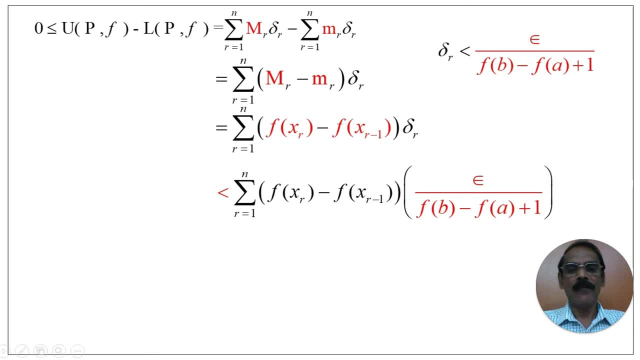 Now, what is the value of sigma R equal to 1 to n, f of xr minus f, of xr minus 1?? To get this value, we are going to keep the value of R equals to 1,, 2, 3 up to n. 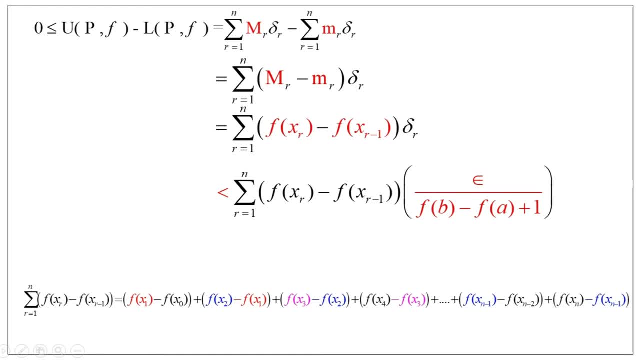 Sigma R equal to 1 to n, f of xr minus f of xr minus 1 is equals to Now put R is equal to 1.. When you keep R equal to 1, f of xr becomes f of x1.. When you keep R equal to 1, R minus 1 becomes 1 minus 1: 0.. 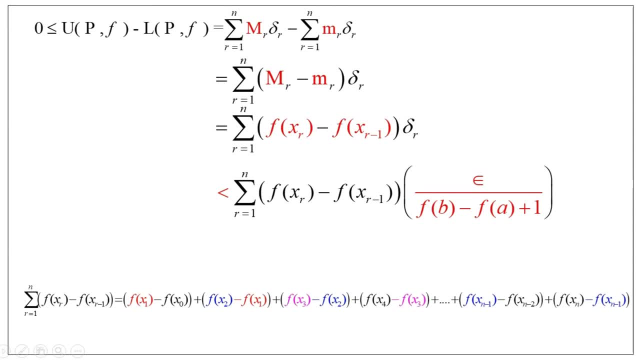 Therefore f of x naught Plus. because we have summation, we write plus here. Now put R is equals to 2.. Therefore it becomes f of x, X2 minus f of x2 minus 1. That is f of x1 plus. 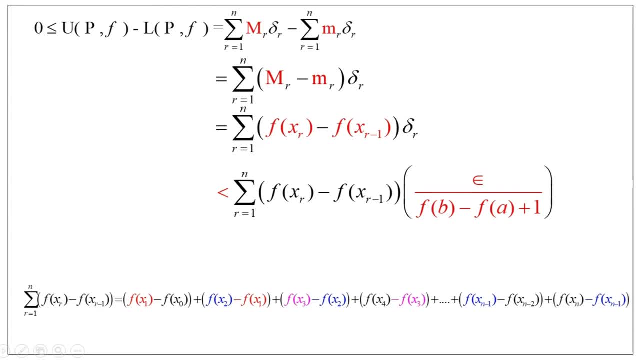 Now put R equal to 3. Then this becomes f of x3 minus. this becomes f of x2 plus. Now put R is equals to 4. Therefore it becomes f of x4 minus f of x3.. So 1. Now put R is equal to n minus 1.. 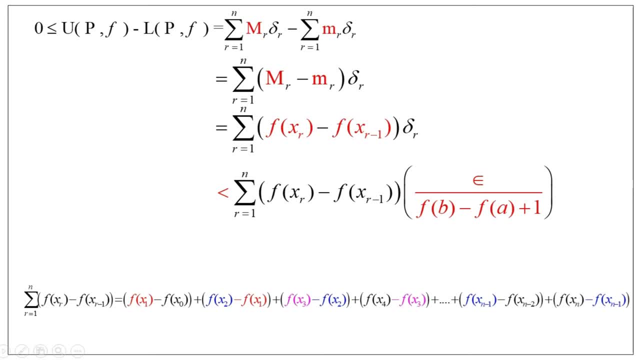 Therefore it becomes f of x minus 1 minus f of xn minus 2.. Plus Now put the last value, namely R is equals to n, Then it becomes f of xn minus f of xn minus 1.. If you look at these terms, 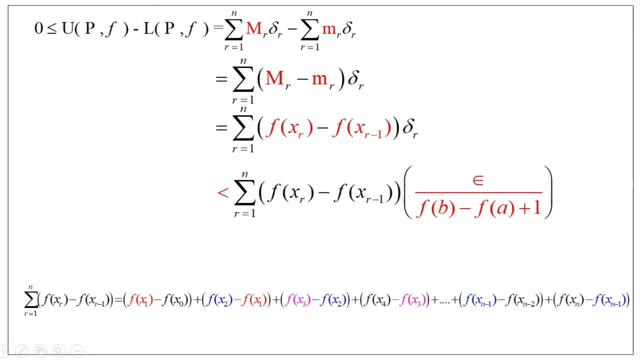 Here you can see f of x1 minus f of x1. So these two get cancelled, Then f of x2. Minus f of x2 get cancelled. Similarly, f of x3 minus f of x3 get cancelled, So 1.. 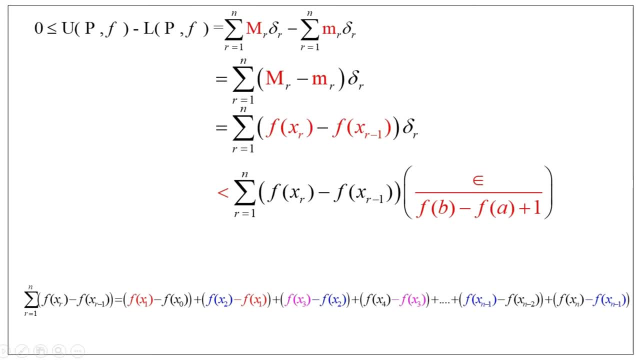 Here f of xn minus 1.. f of xn minus 1 get cancelled, So 1.. Finally, we will get f of xn minus f of x0.. What is f of xn? What is xn value? Xn value is b. 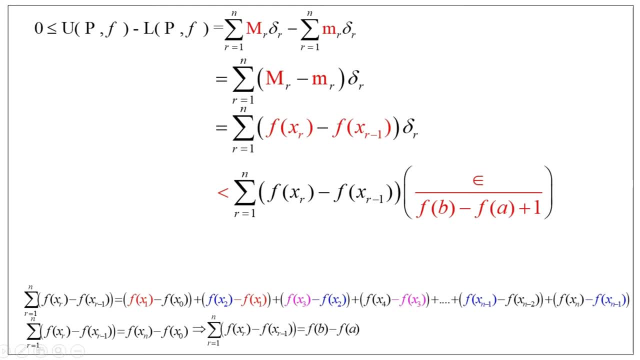 What is x0 value? X0 value is a. Therefore f of xn is equal To f of b, minus f of x0 is f of a. Thus the value of the sum is f of b minus f of a. Therefore, the above expression is equals to: 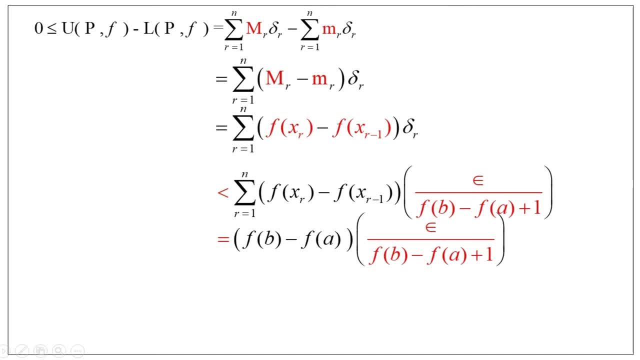 f of b minus f of a Into epsilon by f of b minus f of a plus 1. That is equal to epsilon by f of b minus f of a, By f of b minus f of a plus 1.. Now let us find the. 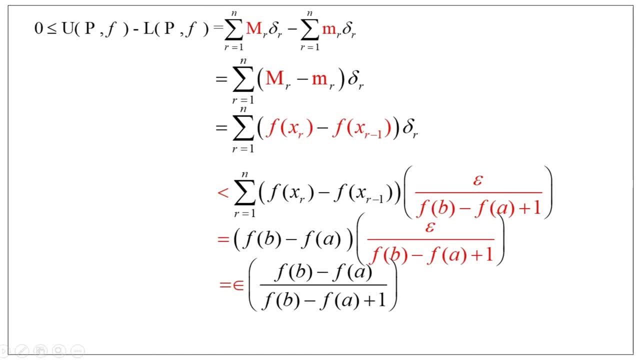 value of f of b minus f of a by f of b minus f of a plus 1.. It is clear that f of b minus f of a plus 1 is greater than f of b minus f of a. f of b minus f of a is positive value. 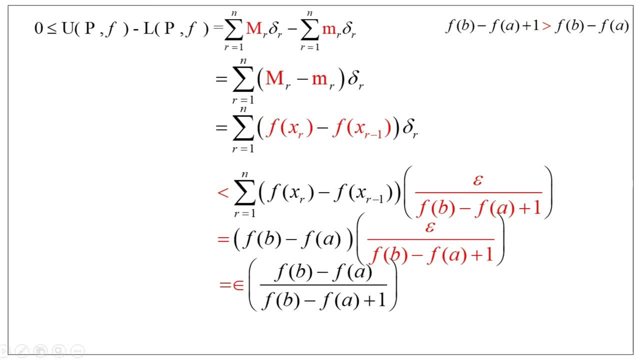 We are adding 1 to the left hand side. Therefore, the left hand side is greater than the right hand side, And this can be written as: f of b minus f of a is less than f of b minus f of a plus 1.. 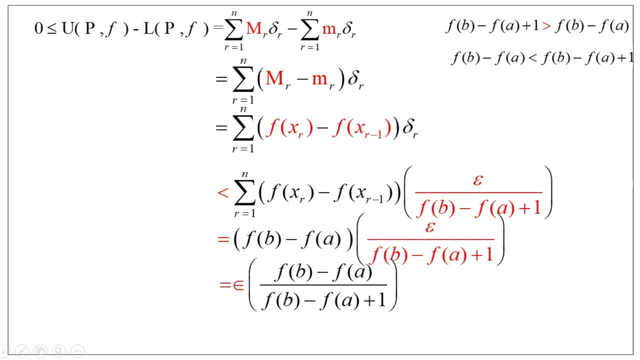 Now bring this f of b minus f of a plus 1 to the left hand side. Therefore, f of b minus f of a by f of b minus f of a plus 1 is less than 1.. Thus the value of this expression is less than 1.. 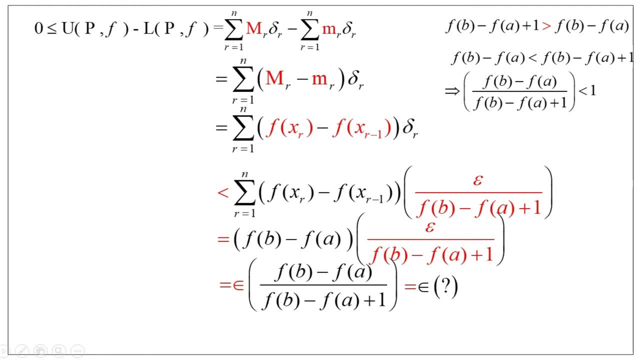 Therefore it is equals to, That is, this expression is equals to epsilon into Its value is Simply less than epsilon. Therefore this equality is replaced by less than, So less than epsilon. Thus, u of b comma f minus l of b comma f is less than epsilon. 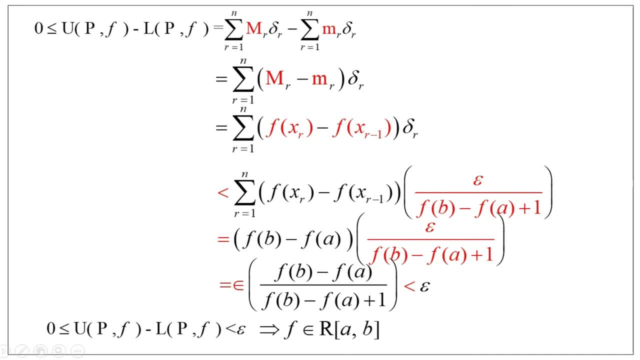 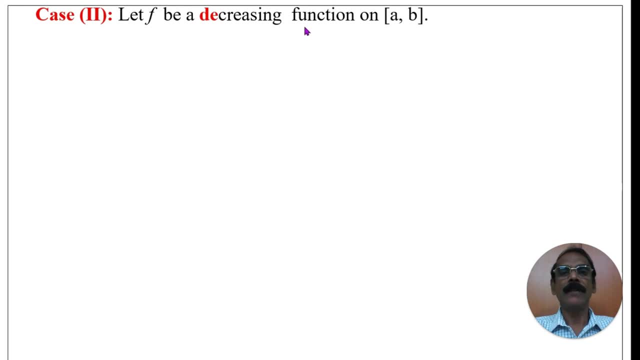 That is f, is Riemann integrable? Case 2.. Let us consider the function f b, A decreasing function. On the closing Reveal a, comma b. This implies, Since f is a decreasing function Minus f is an increasing function. 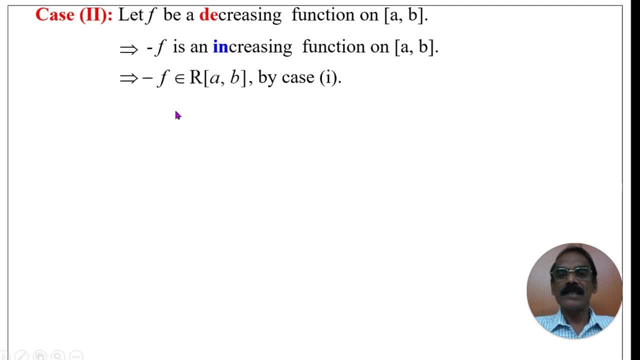 On the closing Reveal a comma b. Just now we have shown that Every increasing function is Riemann integrable, Since minus f is one of the increasing functions Which must be Riemann integrable. Therefore, minus f belongs to R of a comma b. 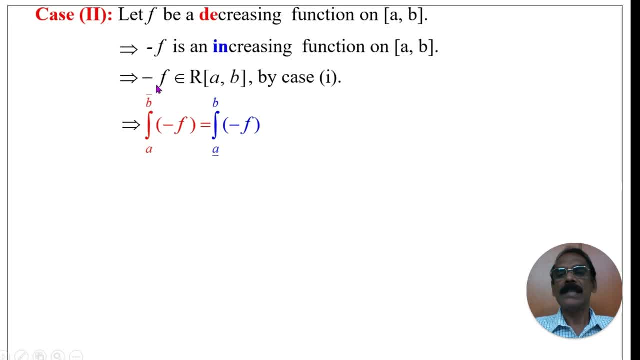 This is by case number 1.. Since minus f is a Riemann integrable, Then the upper Riemann integral of minus f Is equals to lower Riemann integral of the function minus f, That is, integral from a to b. bar minus f is equal to. 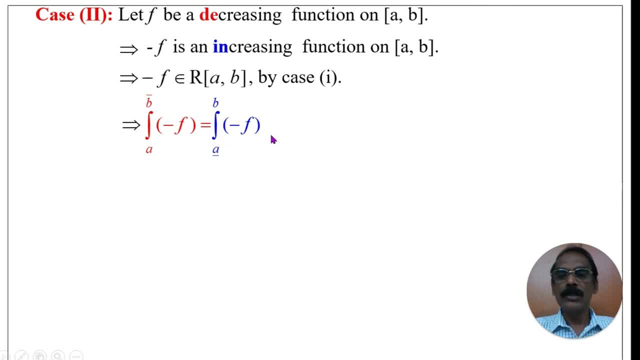 Integral a bar to b minus f. Also, we know that upper Riemann integral of minus f is equals to minus of lower Riemann integral. Similarly, the lower Riemann integral of minus f is equals to minus of upper Riemann integral. 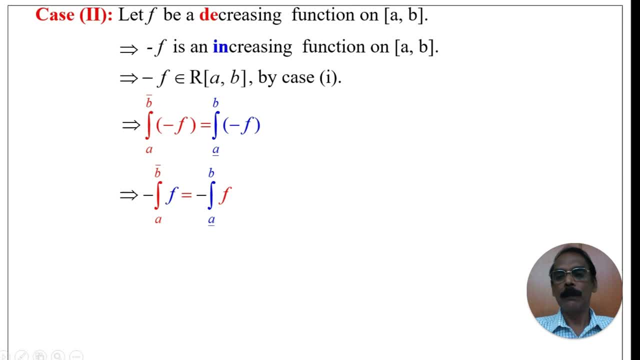 Therefore the next step is minus of a to b bar f is equal to minus a bar. Now cancel this minus sign on both sides. We get integral from a to b. bar f is equals to integral a bar to b f. That is upper Riemann integral of the function f. 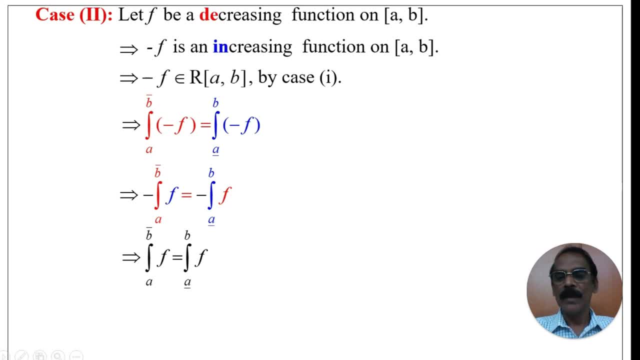 Is equal to lower Riemann integral of the function f. What is the function f? The function f is a decreasing function, That is, the function f is Riemann integral And this decreasing function is Riemann integral. Case 1 says that every increasing function is Riemann integral. 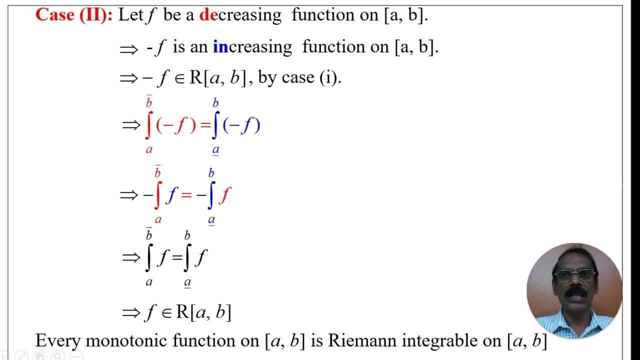 Case 2 says that every decreasing function is Riemann integral on the given closed interval a- b. Therefore we conclude that every monotonic function on the closed interval a- b Is Riemann integral on the closed interval a- b. 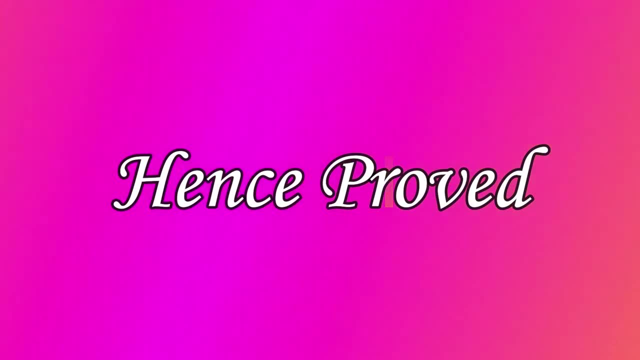 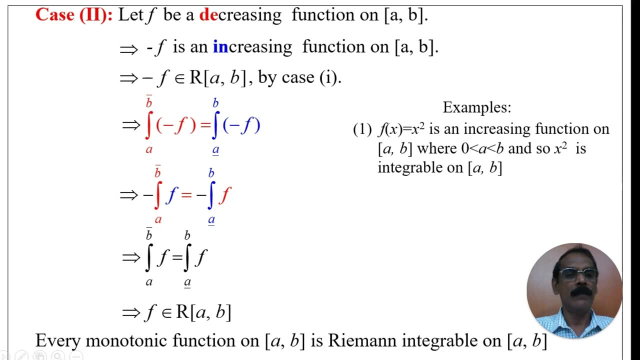 interval a comma b. Examples: f of x is equal to x, squared is an increasing function on the closed interval. a comma b, where 0 less than a less than b and so x squared is integrable on the closed interval. a comma b and f of x is equal to 1 by x is a decreasing function on the closed interval. 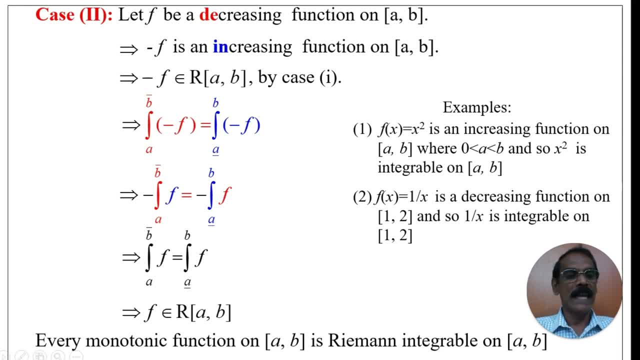 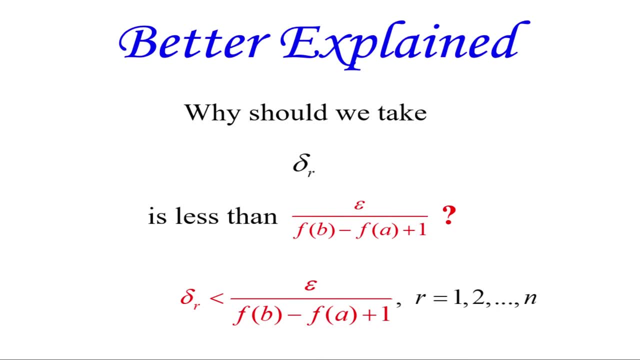 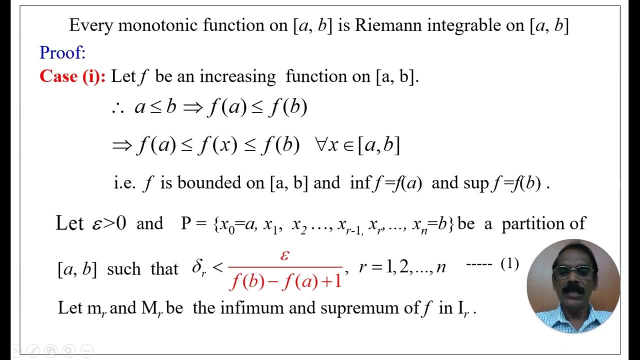 1 comma 2, and so the decreasing function 1 by x is integrable on the closed interval 1 comma 2.. Why should we take delta? r is less than epsilon by f of e minus f of a plus 1? The reason is: 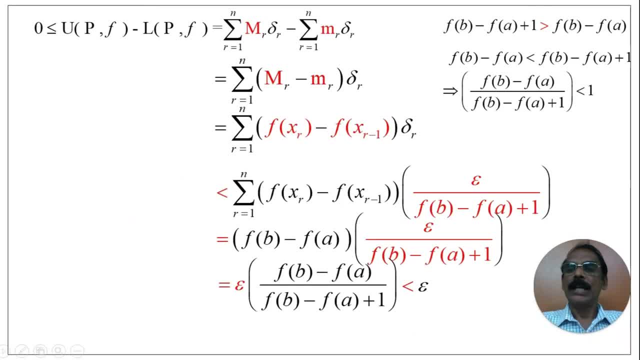 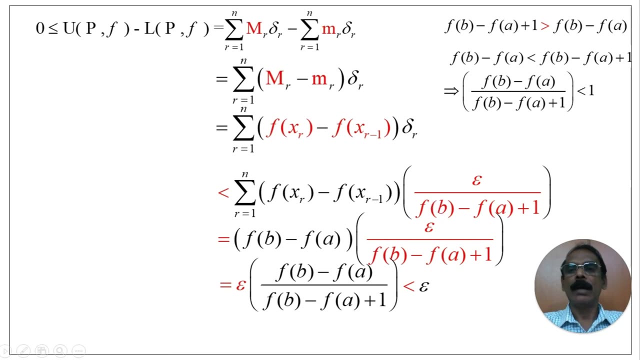 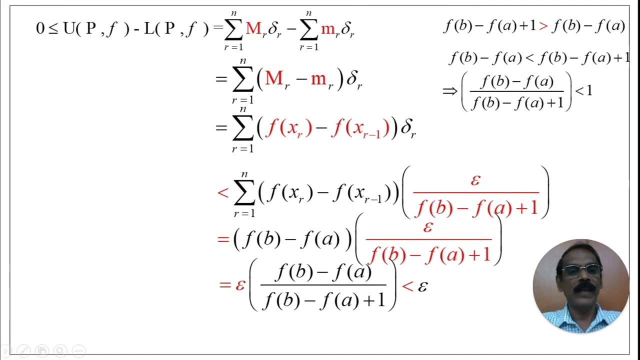 our aim is to show that the difference of upper dot box sum and the lower dot box sum is less than epsilon. How do you get less than epsilon? Up to here the value is same. When we calculate upper Riemann integral minus lower Riemann integral, we get this sum is f of b minus f of a into delta r. Now our aim is to get less. 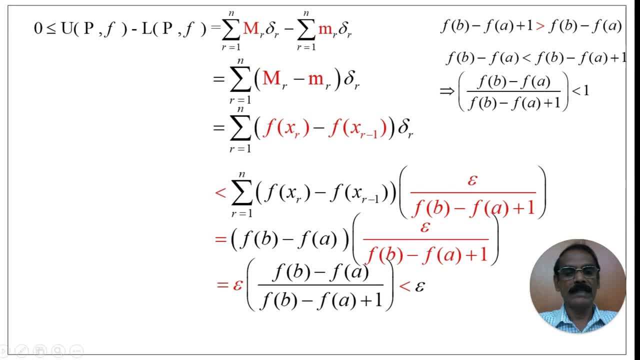 than epsilon. Since this sum is f of b minus f of a, to get epsilon we have to take: delta value is equal or less than epsilon by f of b minus f of a. But here we have taken epsilon by f of b minus f of a plus 1, so that we get directly its value is. 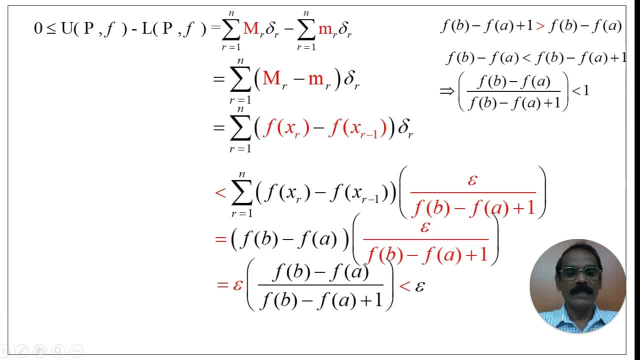 less than epsilon. The value of f of b minus f of a by f of b minus f of a plus 1 is less than 1 and hence we get this is less than epsilon, To make the difference of upper Riemann lower Riemann. 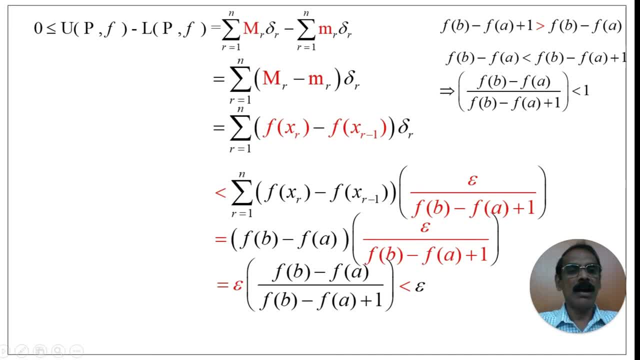 less than epsilon. we are taking delta r value is less than epsilon by f of b minus f of a plus 1..